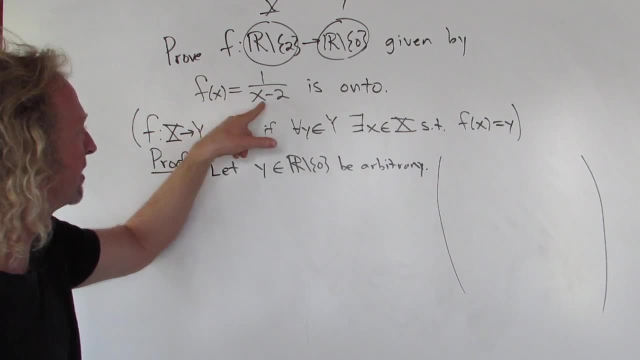 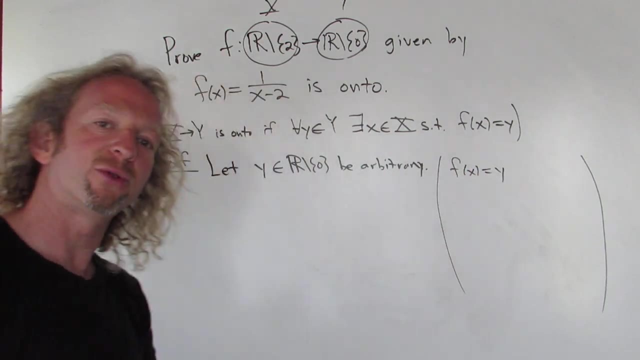 we want little y in this set, so that f of X is equal to Y. so we need f of X to be equal to Y. so, again, this is not the proof of working backwards, but this is how you figure out the proof, which is really really important. so f of X is 1. 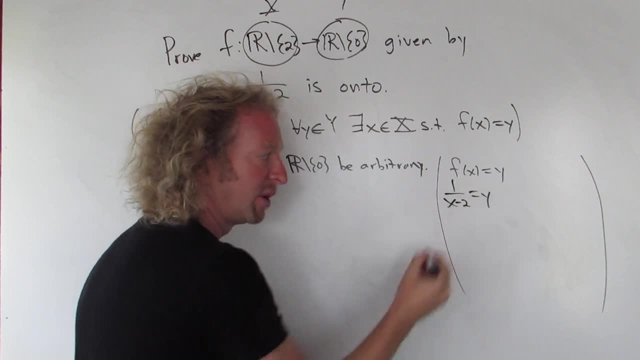 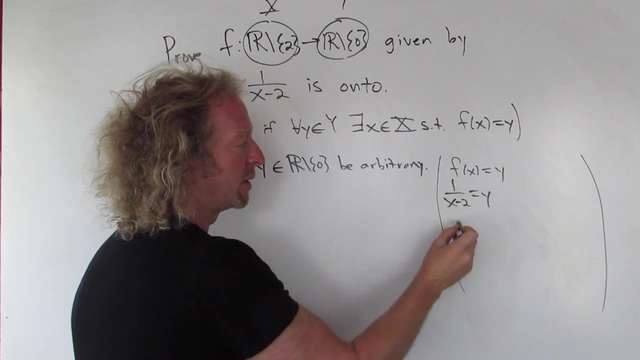 over X minus 2, that's equal to Y. we can multiply both sides by X minus 2, so you do X minus 2, X minus 2. I won't write it because I'm running out of time, I'm running out of room. so you would get 1 equals Y times X minus 2, basically. 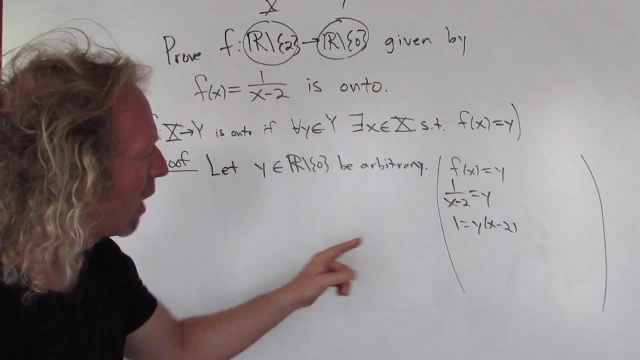 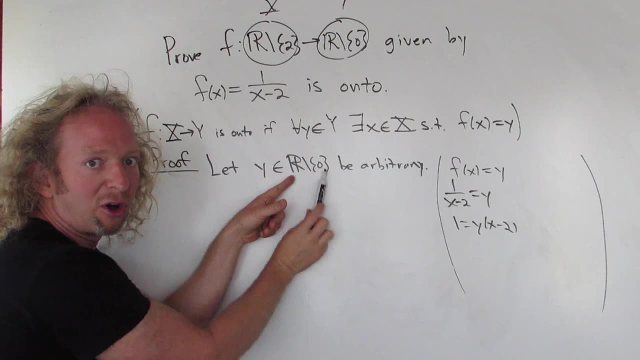 multiplied by X minus 2 and they cancelled. okay, I didn't show that step and we're looking for X so we can divide by Y. note that Y is not 0 because it's in the set of real numbers, set minus 0, so it's all the real numbers except 0. so 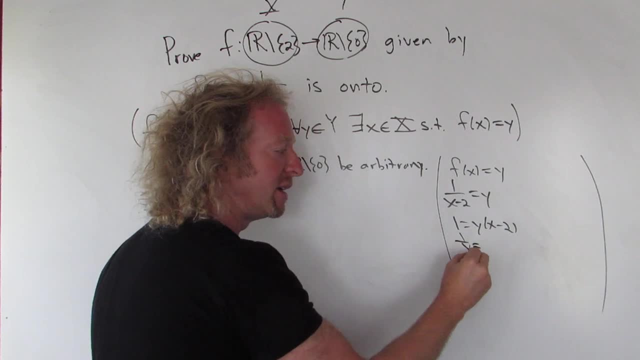 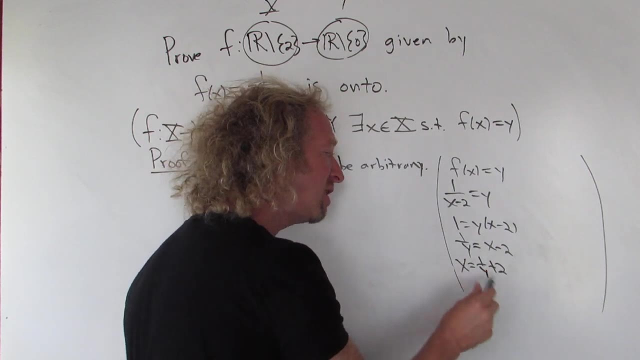 we can divide by Y super key, so 1 over Y is X minus 2. then you can add 2 to both sides, so you get X equals 1 over Y plus 2. so that's gonna be the little X we want. we need to make sure. 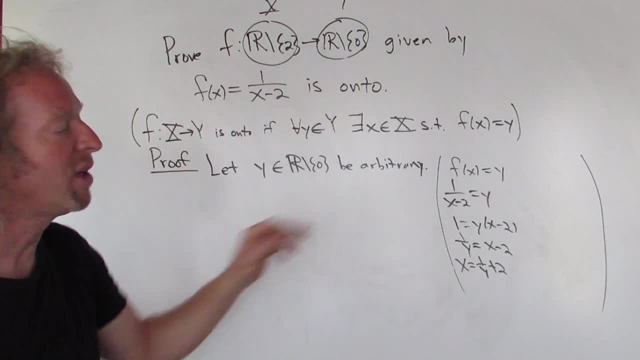 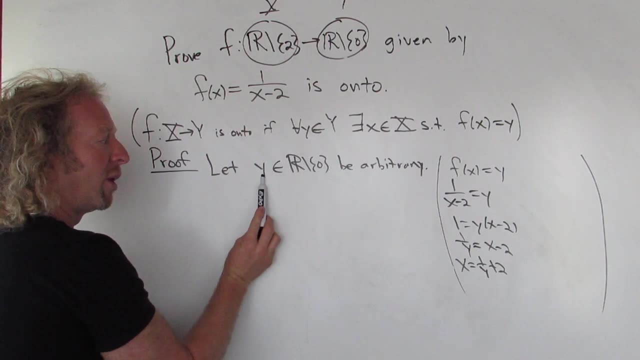 that little X is in this set. right, we'll do that in the proof. we'll deal with that in the proof. so now we're going to go back to our proof. okay, so we start our proof by letting little Y be in this set, which is this set here, the? 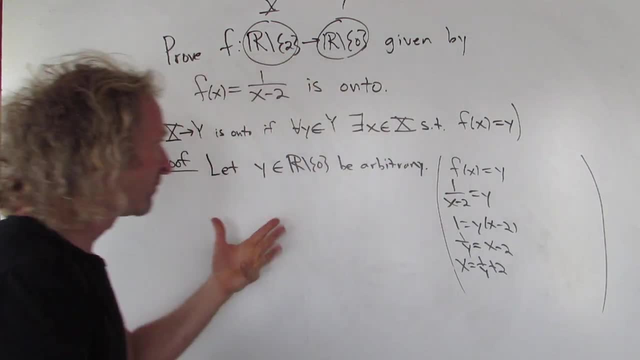 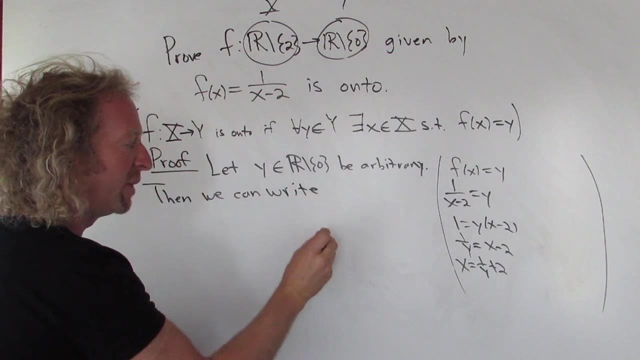 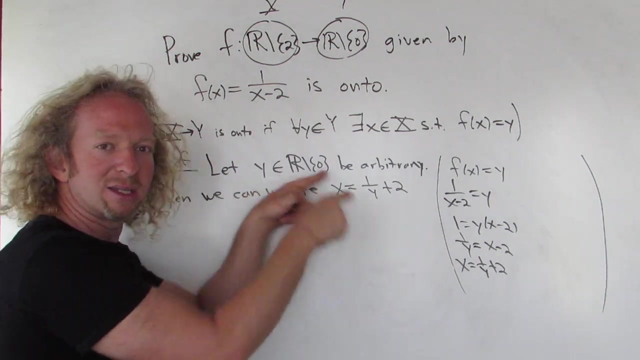 arbitrary. now we have to show the existence of little X. so then we can write: why am i writing that? ah, we can write: little X equals 1 over Y plus 2. we can write it because it makes sense, because Y is not 0, Y is in the set, so it's not going to be 1 over 0, so we can write that. so we can. 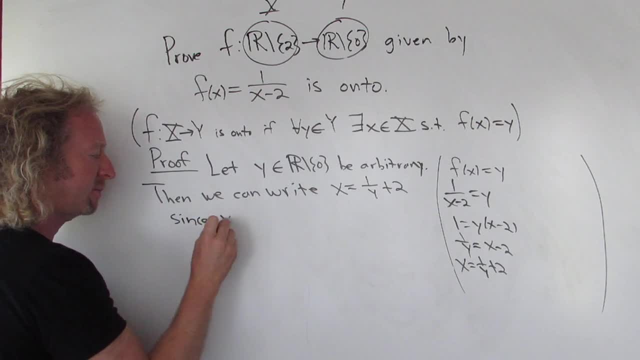 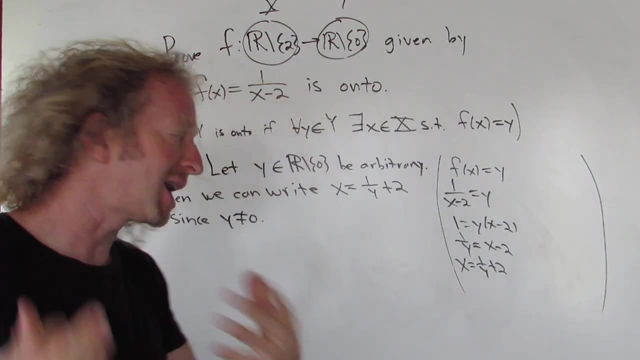 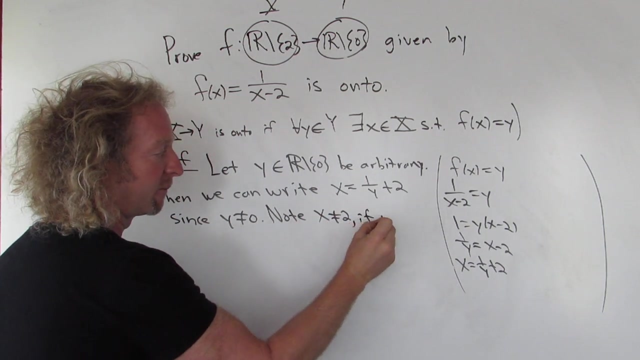 write that since Y is not 0, now we have to explain why it's in this set right. Y is in capital X. so to explain why it's not equal to 2. so note X is not equal to 2, if it were, or if it was, we would have- let's do a proof by contradiction- said that was equal. 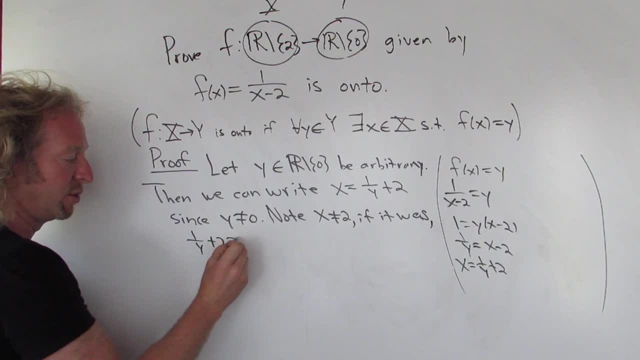 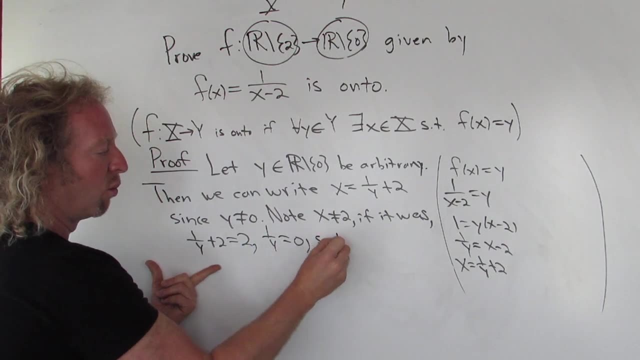 to 2. have 1 over y plus 2 equals 2, right x equals 2.. Well, you would subtract 2, so you would get 1 over y equals 0.. Multiplying by y, you would get 1 equals 0.. That's a contradiction, okay, You? 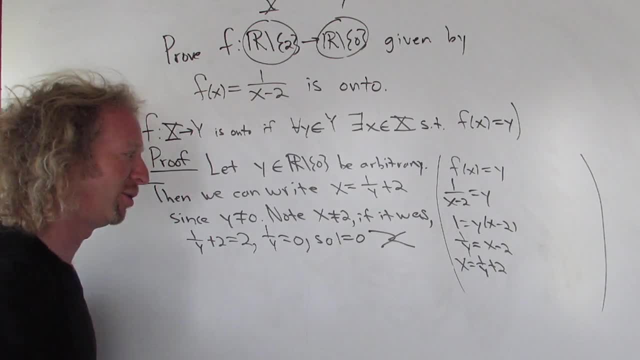 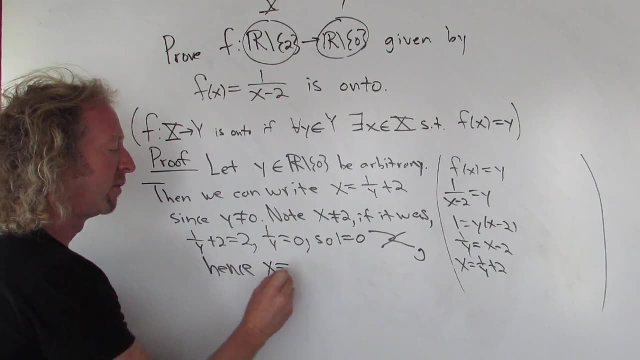 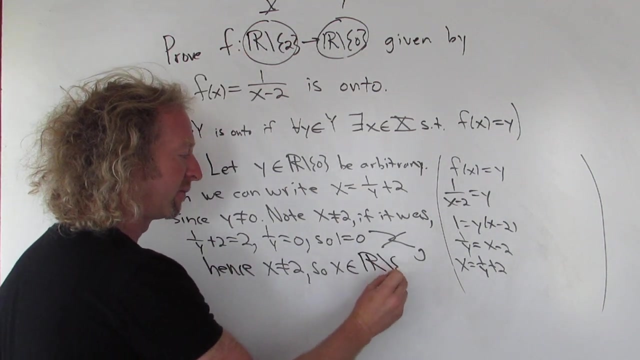 can use that for contradiction. I saw that one time somewhere, I thought it was cool, so I stole it. Contradiction Hence. hence, x is not equal to 2.. So little x is indeed in this set here. right, Beautiful stuff. okay, Now we're almost done. Now we just have to show that f of x is. 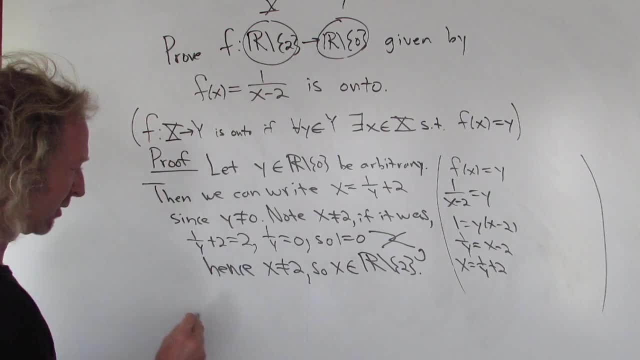 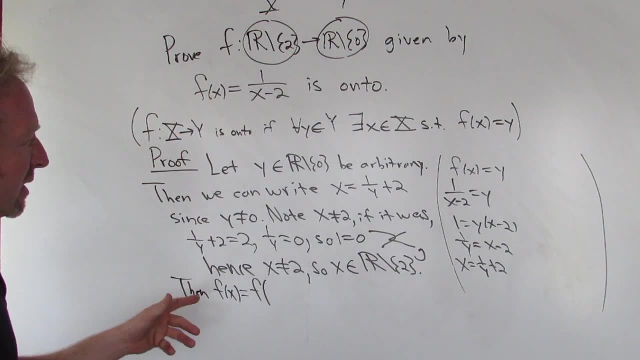 equal to y. So it really is a beautiful argument. So now? so then, hopefully you can see f of x is equal to f of well, x is 1 over y plus 2.. So f of x is 1 over x minus 2.. Now you just replace your x with 1 over y plus 2, so it'll be. 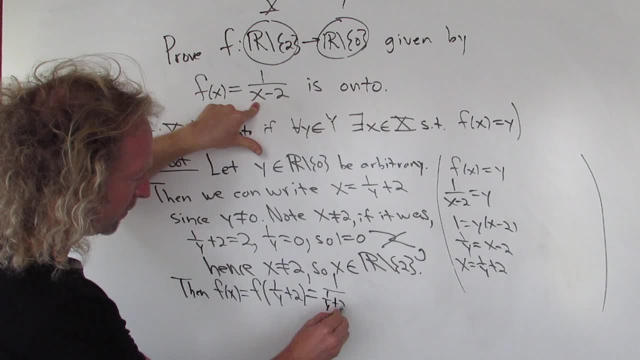 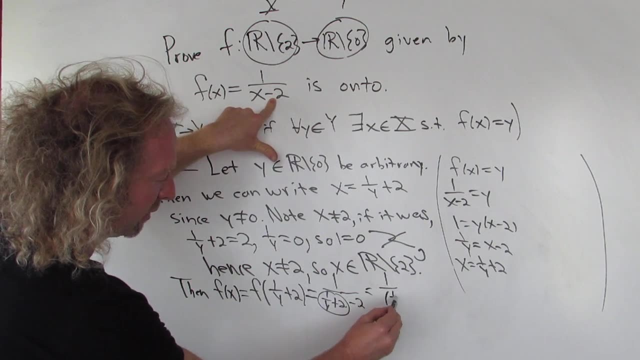 1 over x, So it's 1 over x plus 2.. 1 over x, 1 over y plus 2, that's your x, right there. okay, this is your x and then minus 2, these cancel, so it's 1 over 1 over y. when you take 1 and you divide it by 1 over y, you 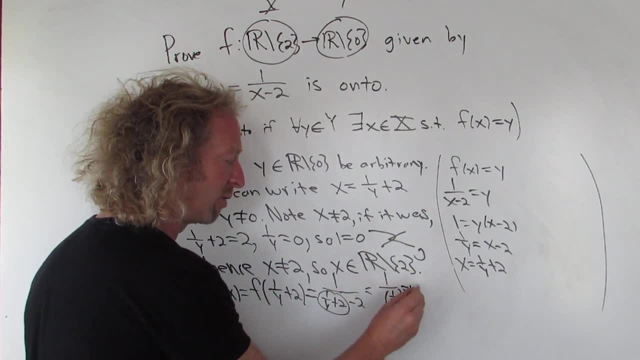 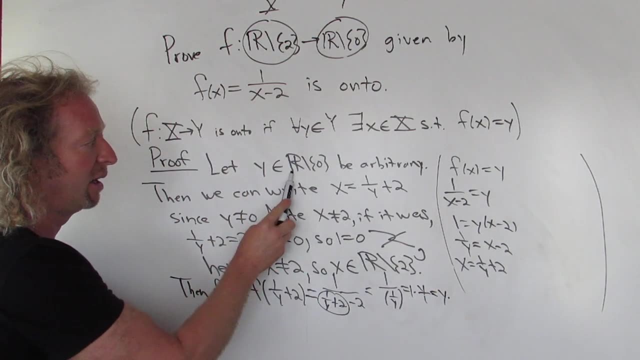 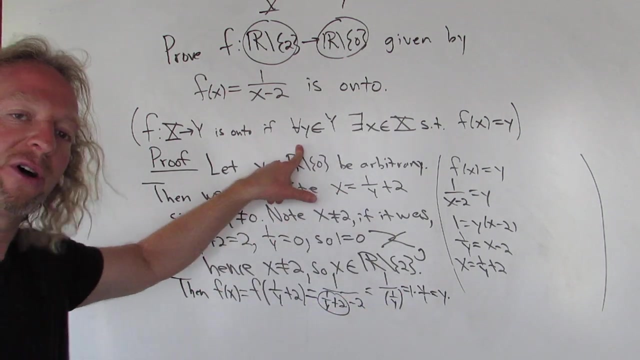 really multiply by the reciprocal. so it's 1 times y over 1,- let's be really pro about this- which is equal to y, boom. so we took any little y and this set. we found an x. we showed it was in this set and then we showed f of x is equal to y. so for all little 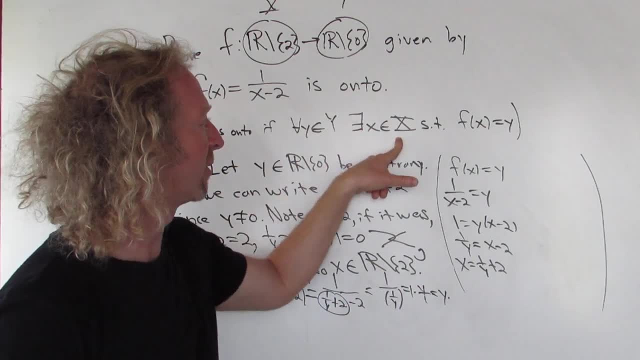 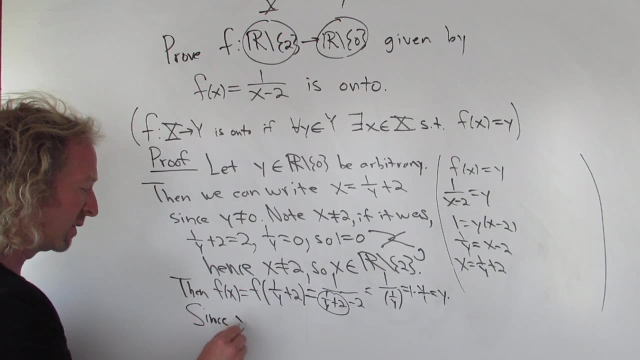 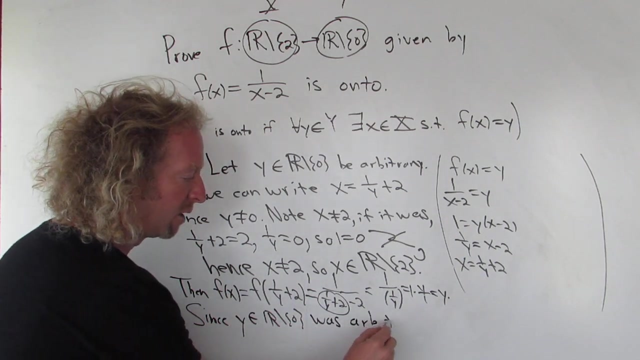 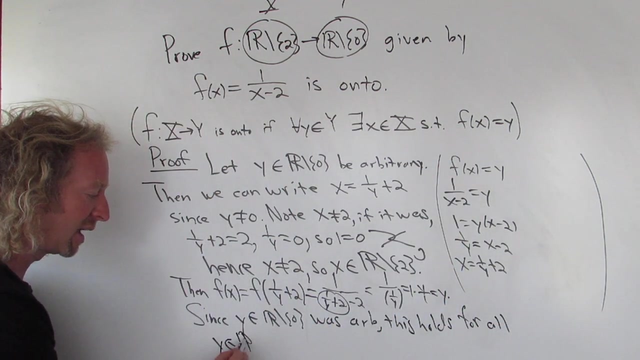 y in capital y, we found that there was a little x in capital x, such that f of x is equal to y. if you want to be really thorough, you can say something like: since y in this set was arbitrary, this holds for all right, for all, for all little y in this set you. 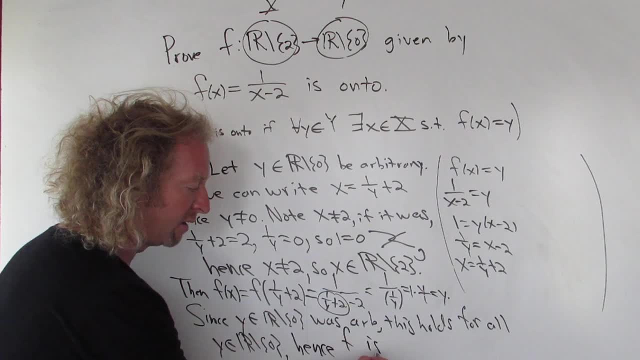 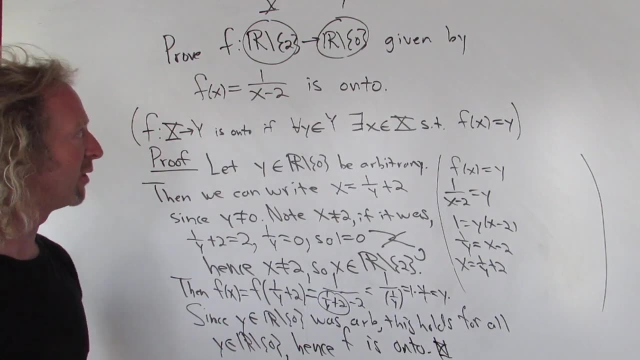 know. hence f F is onto is a surjection and that completes. that completes the proof. so that's a formal proof. hopefully someone out there is working on this stuff, if you are awesome, right, and hopefully that makes sense, that's it.